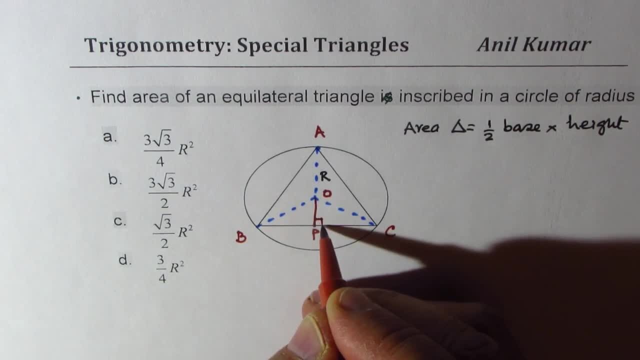 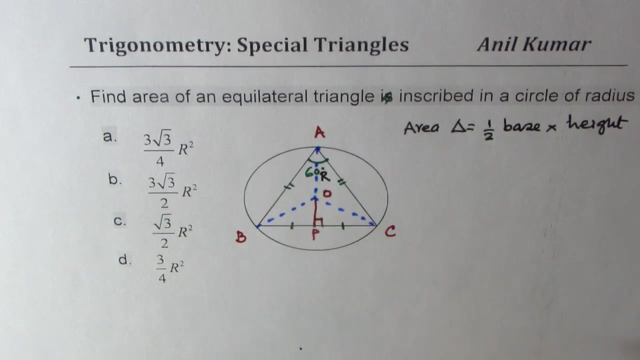 As p, which is perpendicular to the base. Now, each side is equal, right? But this will be like half of that. right Now, how do we find the side of the triangle? Well, we know that the total angle here is 60 degrees, So each angle is going to be how much At the base? this is 30 degrees, right? 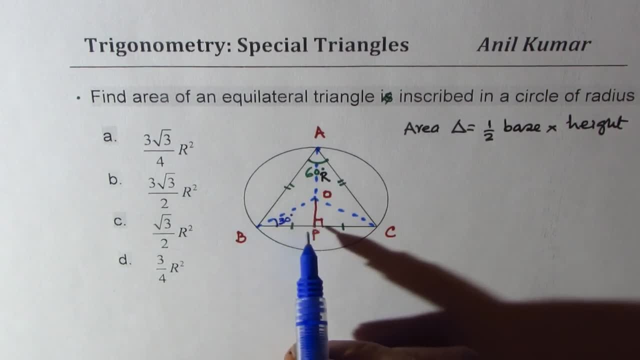 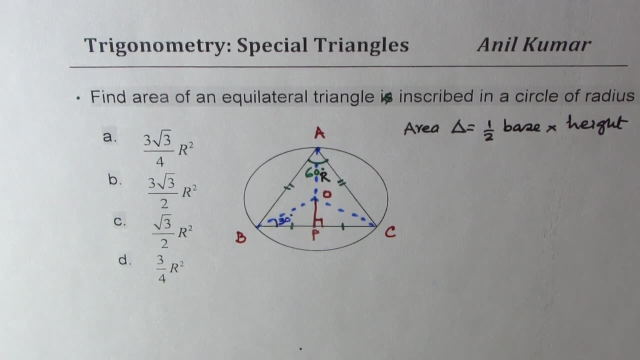 So these angles are 30 degrees. So what we have here is a 30-60-90 triangle, correct? So we can solve with 30-60-90 triangle. So we'll take the special triangle which is 30-60-90 and then do this question without calculator. So that is kind of important. 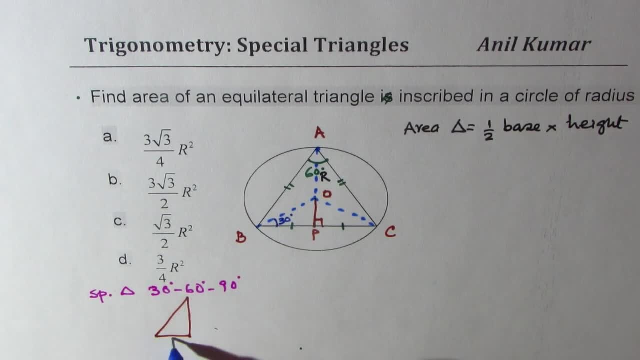 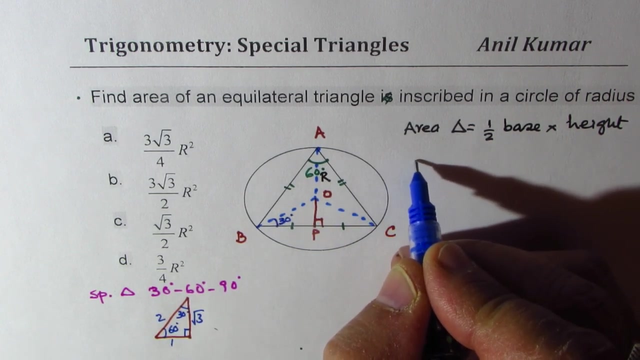 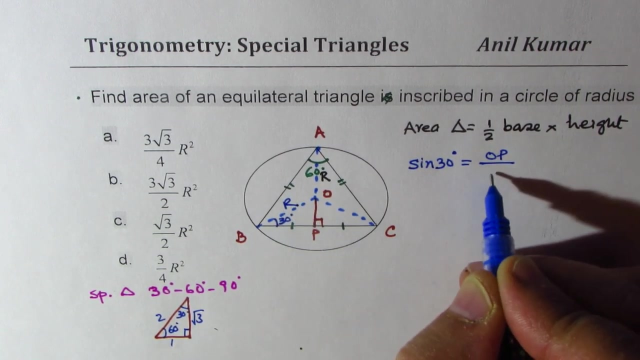 In trigonometry these are very important triangles to always consider. Ratio of the sides will be as shown, And that is 30 degrees. So if I want to find op, then we know that sine of 30 is equal to op over. that is also r right. 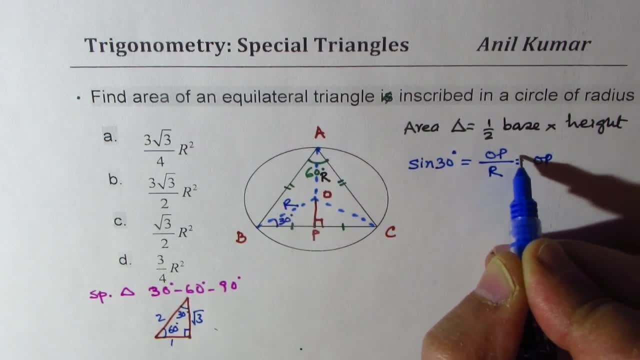 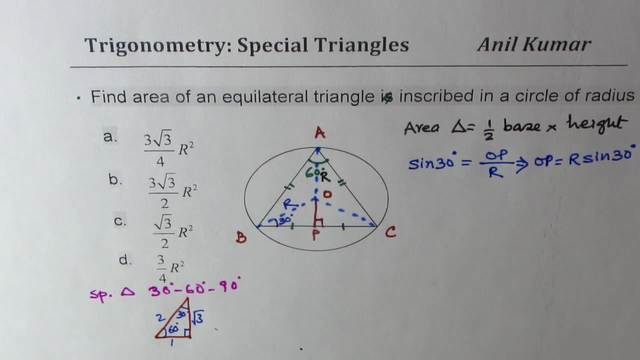 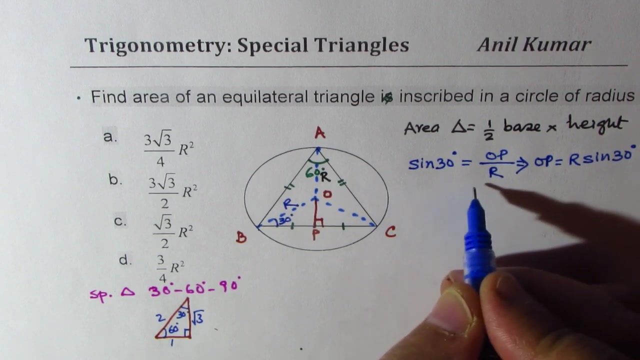 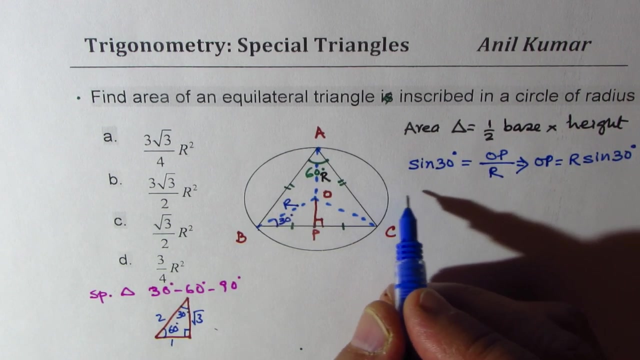 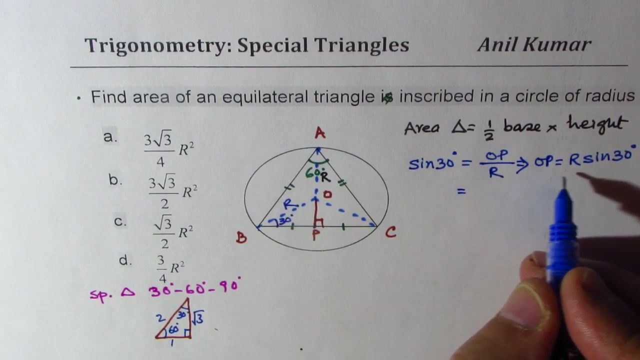 So op is equal to r. So op is equal to r sine 30. Perfect, Now what is bp? equals to Cosine 30 will give us bp right, So let's write. we can write down this value also: Sine 30 is half, So we get op equals to half. 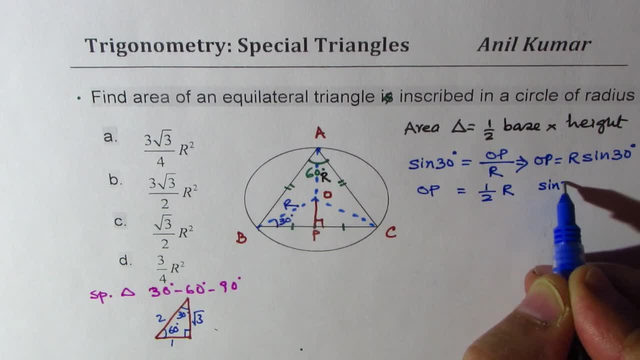 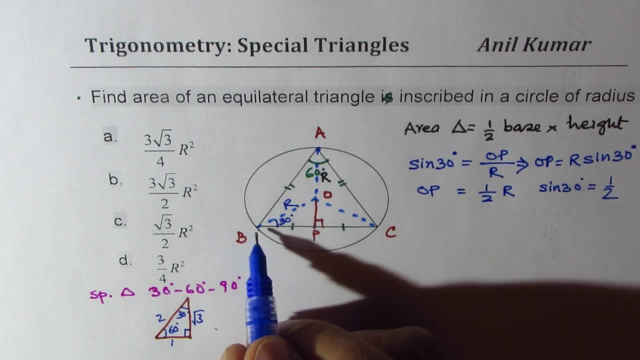 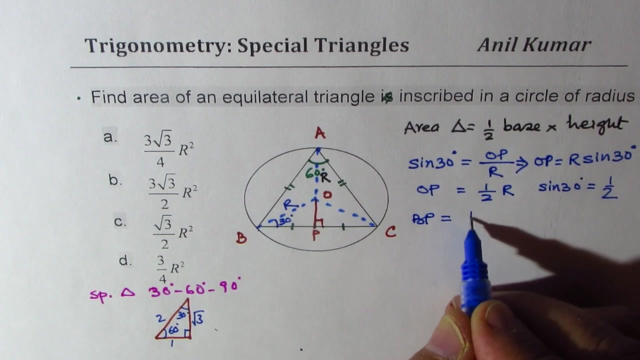 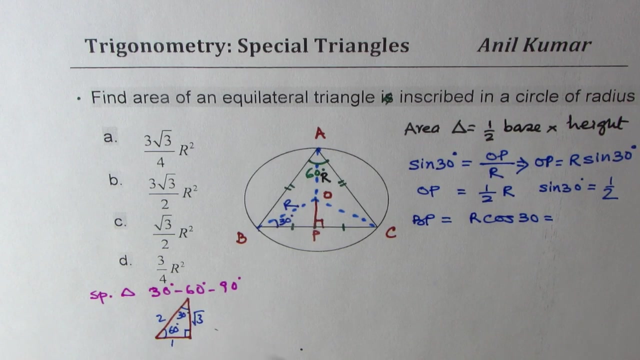 So half of r, Since sine 30, is equal to half right From this triangle. okay, As far as bp is concerned, bp is the cosine of 30, right? So it is r times cos of 30, which is equal to cos of 30, square root 3 over 2.. So it is square root 3 over 2.. 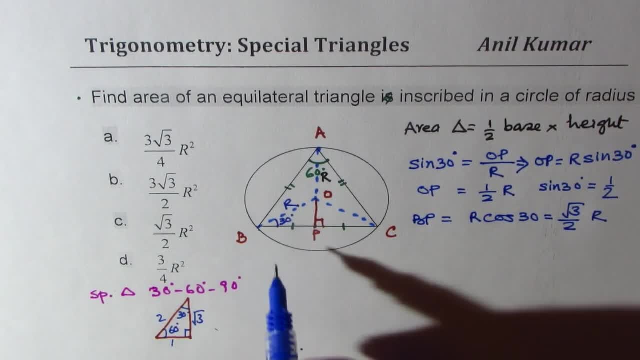 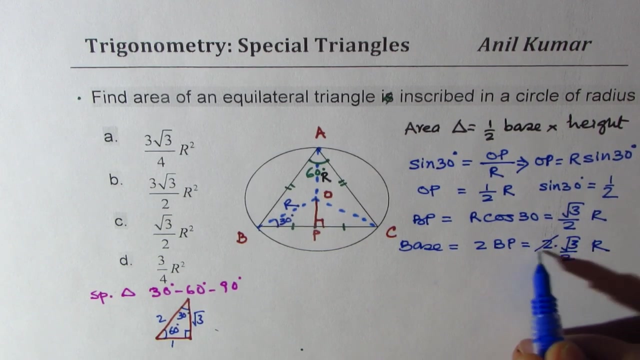 Times r. But the base is how much Base is 2 times bp, right? That means it is 2 times square root, 3 over 2 times r. So 2 and 2 cancel, right, So it is square root 3 r. So what we have here is that the base. let me rewrite this So we have height ap. 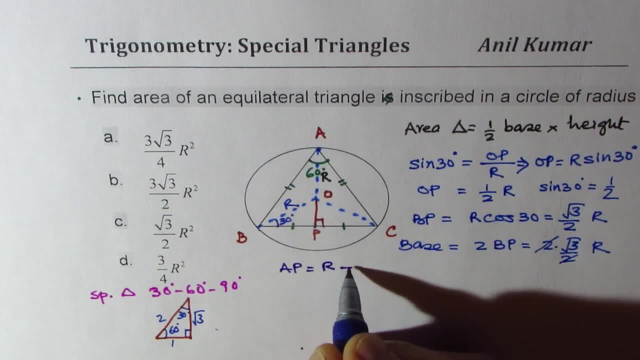 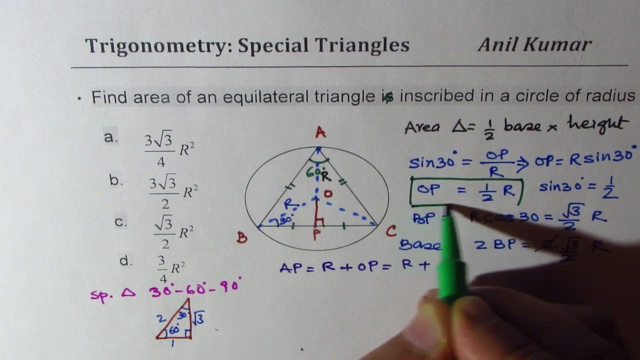 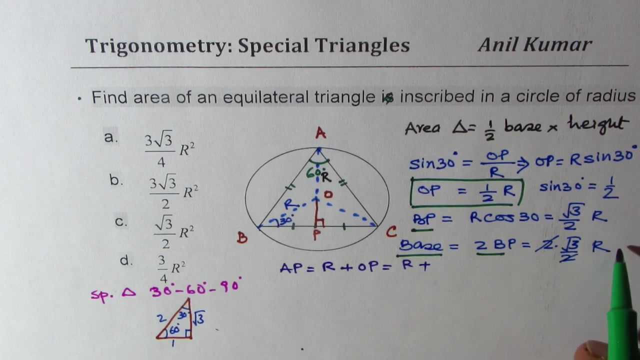 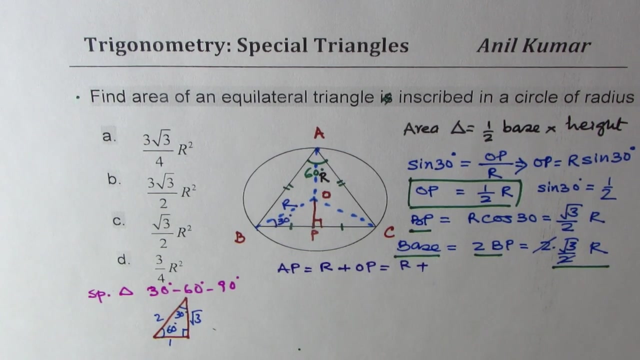 As equal to r plus op, which is r plus op is half r, right. Let me highlight this portion- And bp and the base is 2 bp, which is square root, 3 r. Okay, So what we have here is that a to p is r plus op and op is half r, right, Which is 3 over 2 r, Is it okay? 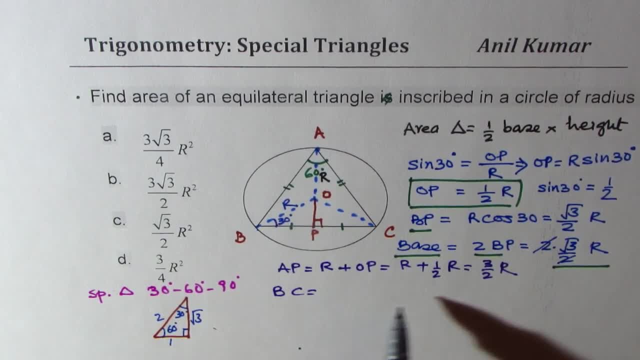 And bc, which is the base, is equal to square root 3 r. So area is how much Area is half of product of these two. So we have 3 over 2 r R times square root 3 r, correct. 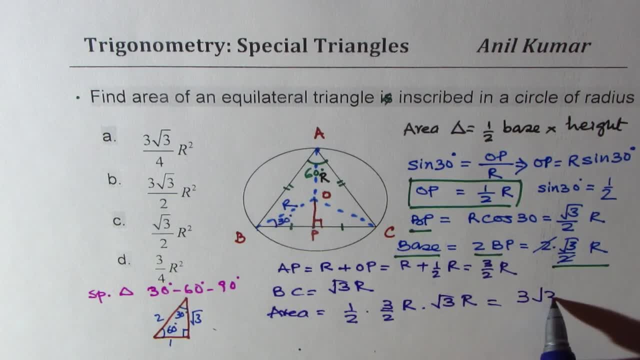 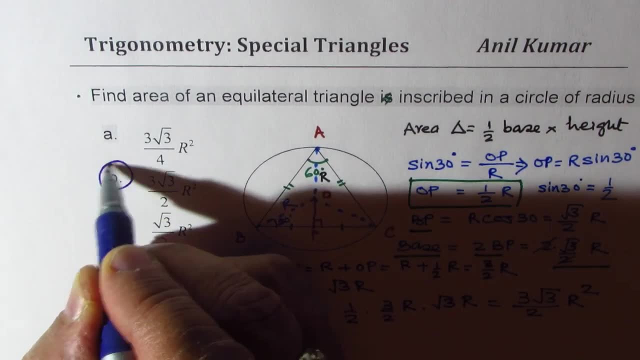 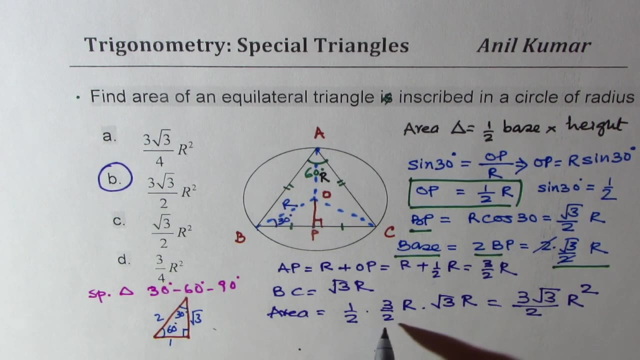 So if you multiply you get 3 square root, 3 over 2 r square, which is option b for us. Sorry, I didn't write this half here, So we have to multiply with this half also. So it is 1 over 4, I'm sorry. 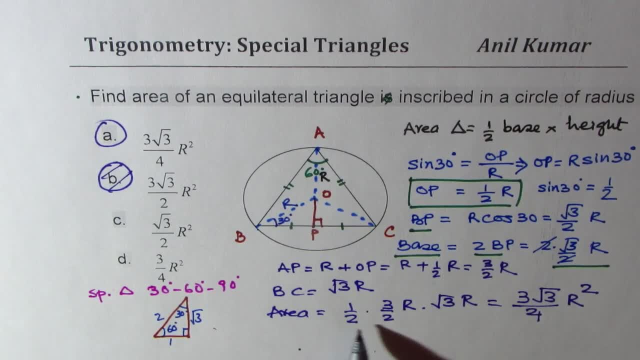 So it is. formula is 3 square root 3 over 4.. half times this, 2 times 2, is 4 right, and 3 square root 3, so forgot this. so it is as you can see. if you multiply this, you get 3 square root 3, r squared. divided by 2 times 2, 4 right. so this is.